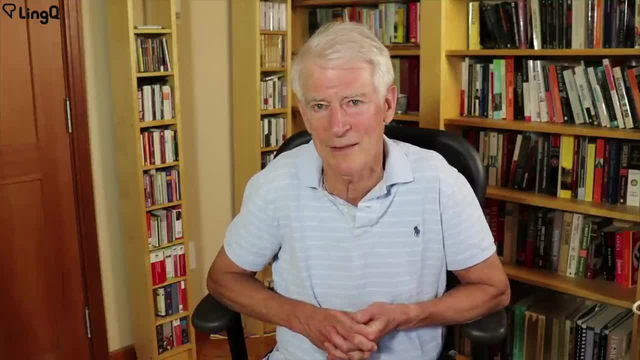 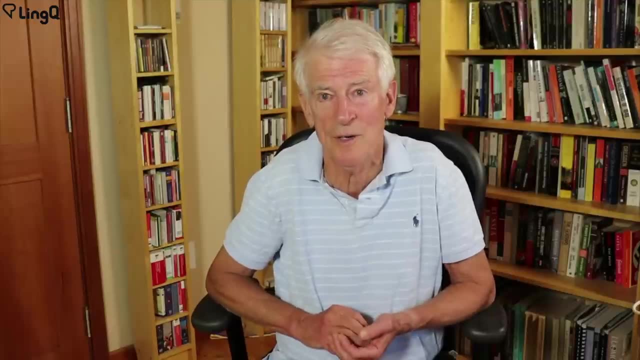 have trouble reading in the language they're learning. is there a way to break that um kind of vicious circle? Well, first thing is, as I just indicated, to be a good reader. to improve your reading comprehension, you have to read a lot. Okay, But let's. 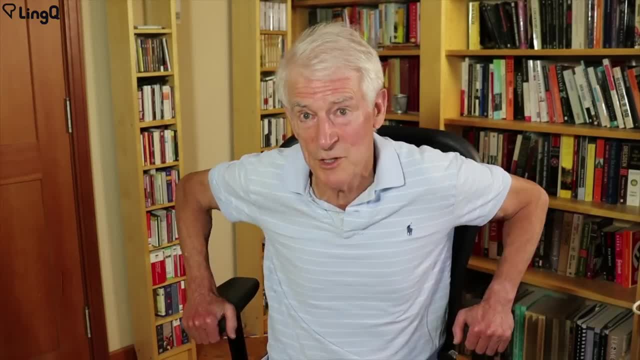 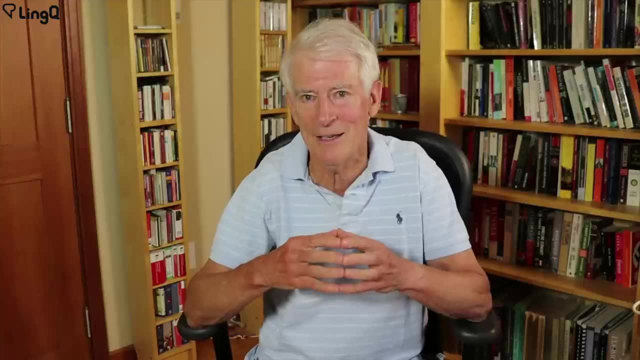 say you have trouble reading. It could be for any number of reasons. First of all, if you're reading in a foreign language, you're not used to reading in that language. You may not be used to reading in the um, the script you know. but 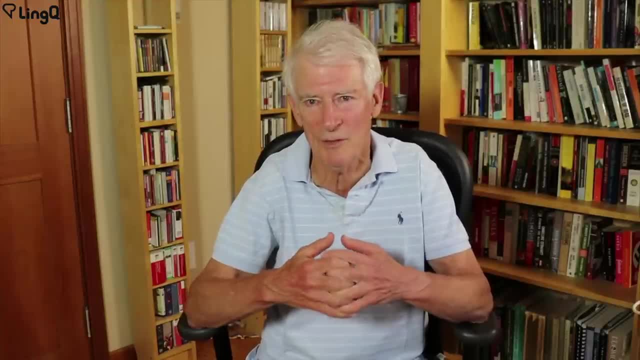 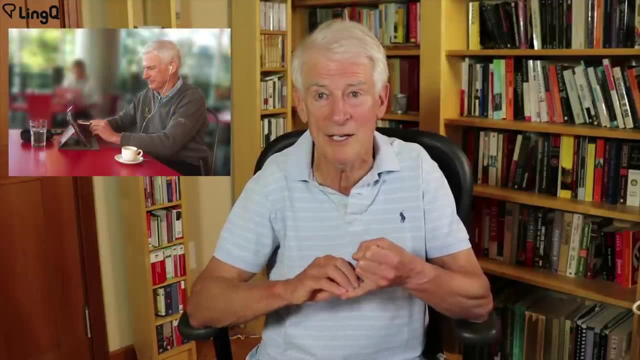 there again: the only solution is to do more of it. You just have to do more of it. But the other things that I find helpful are listening. Okay, Listening combined with reading is very powerful. I find that if I read something, you 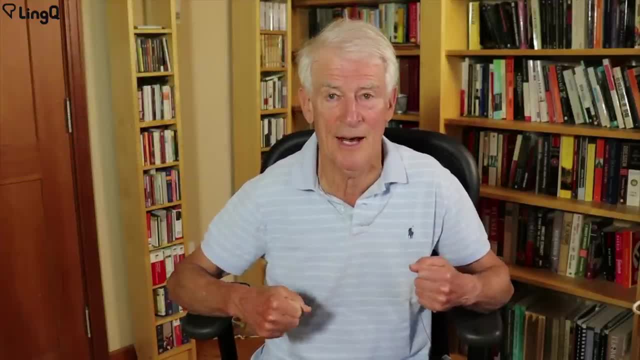 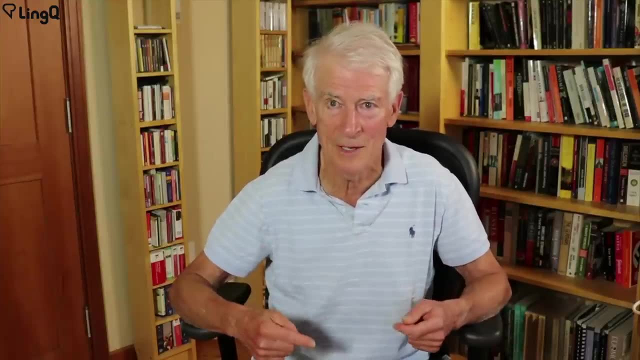 know, without like, without preparation, I have more difficulty reading it. If I can listen to it first, I have an idea of what's there. I have some momentum- Momentum even in so far as the intonation is concerned, then I do. 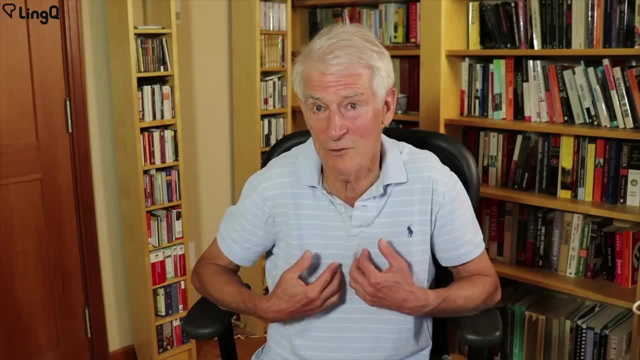 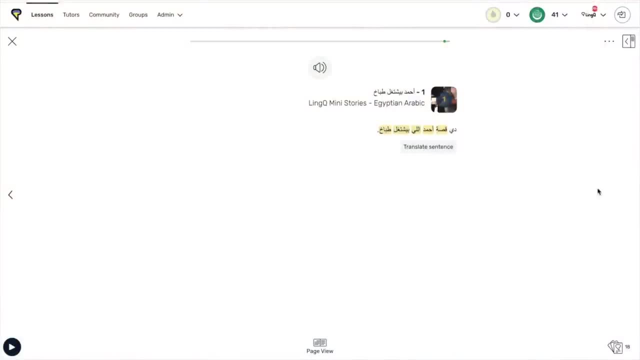 better when I go to read. Also, in languages where I have trouble reading, like Arabic and Persian, I use LingQ and I go in sentence mode so that I might go through the lesson once in sentence mode and then again in in lesson mode. But it it just. 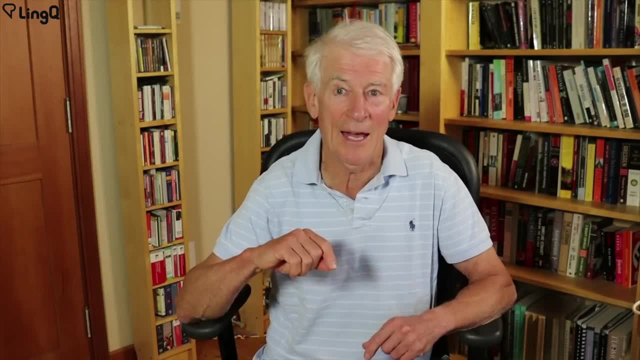 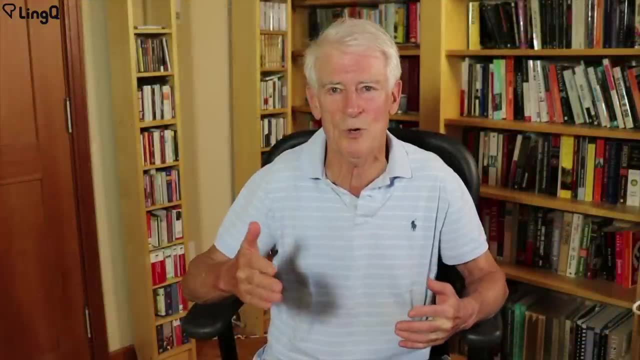 helps me to focus in on one sentence at a time. And then, of course, in order to be able to have good reading comprehension, you need a large vocabulary, because every time you come across a word that you don't know, it's it. 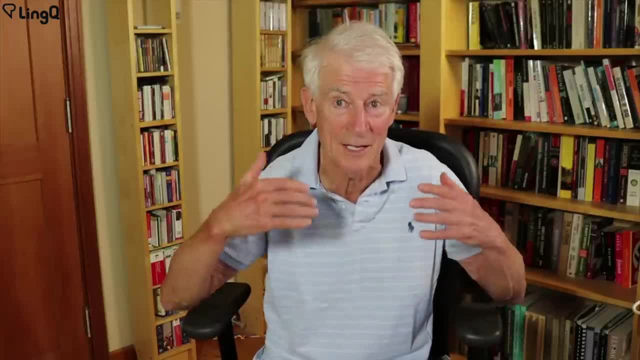 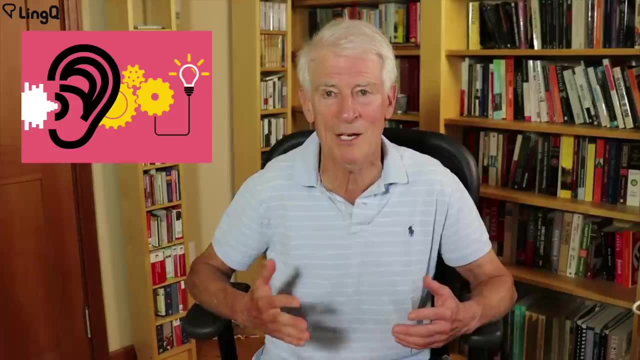 disturbs you. You're, you've got a certain flow and you've got meaning And ideally you want the meaning to flow into your brain without you having to translate in your own lang, into your own language, And every time you hit a 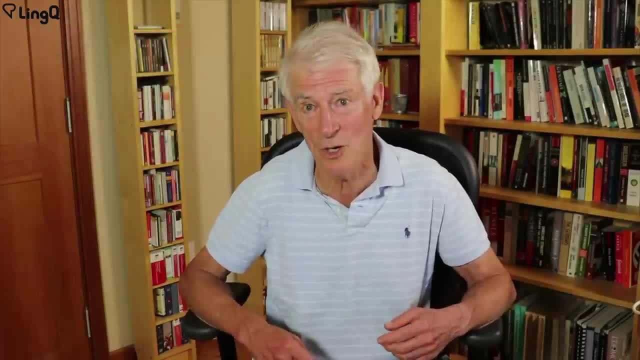 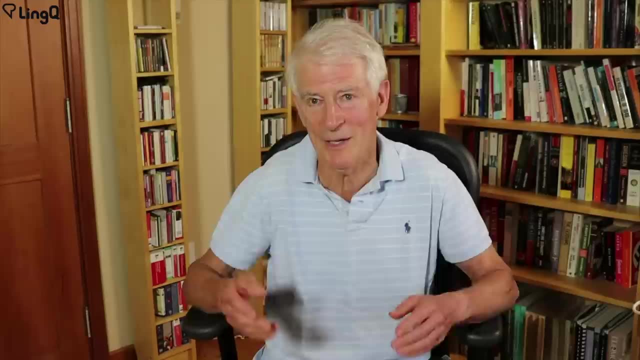 word you don't know. It slows you down. You got to look up the word. you've lost that. that, uh, momentum. So building up vocabulary is extremely important, but in a way it sort of gets back to the same thing. In other words, the more you read the 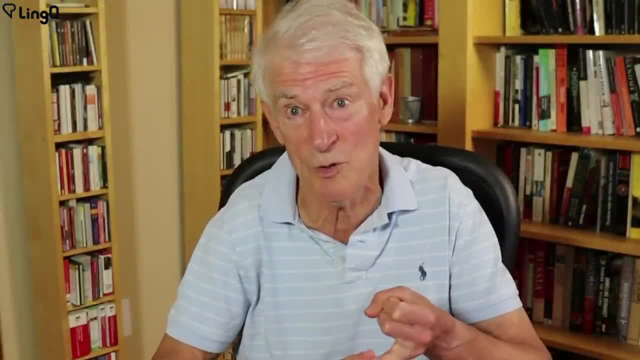 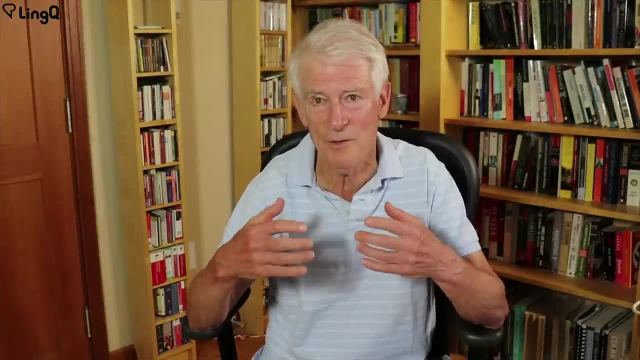 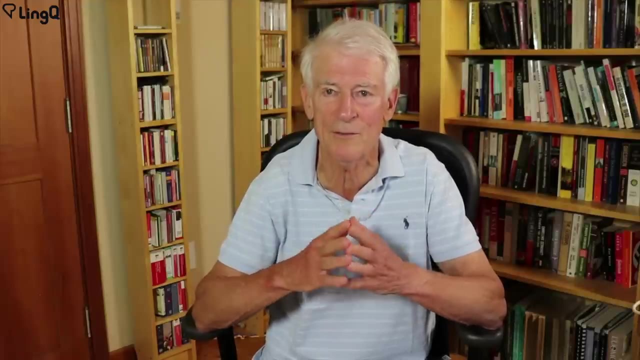 better you read. the more you read, the more words you acquire. the more words you acquire, the better you read. So it's all a virtuous cycle. You have to continuously sort of put yourself in front of reading material and also I would suggest you vary the difficulty level between challenging material. 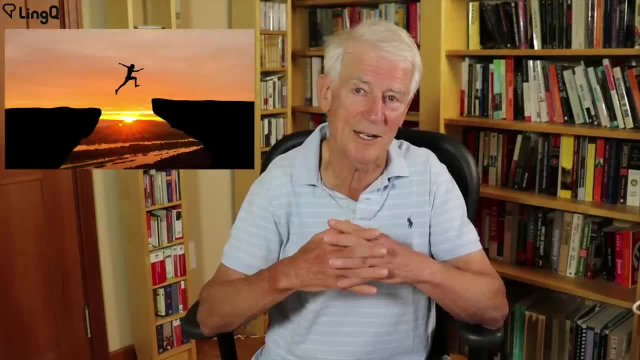 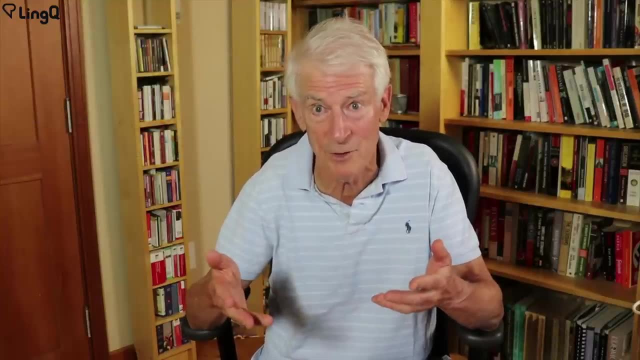 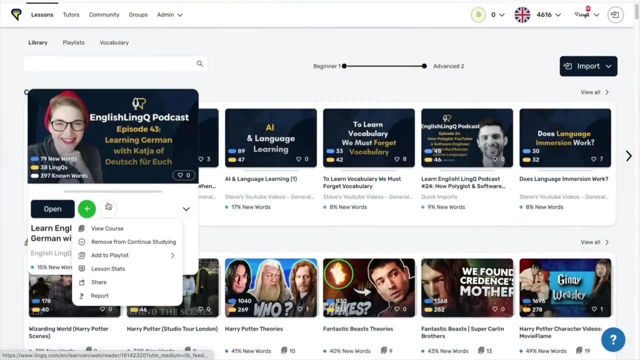 which might have a lot of new words and easy material that has very little in the way of new words. I have found that, since my goal is to become a fluent reader in whatever language I'm learning, but at the same time to acquire more words, I have found that 15% unknown words, as we count them at LingQ, is kind. 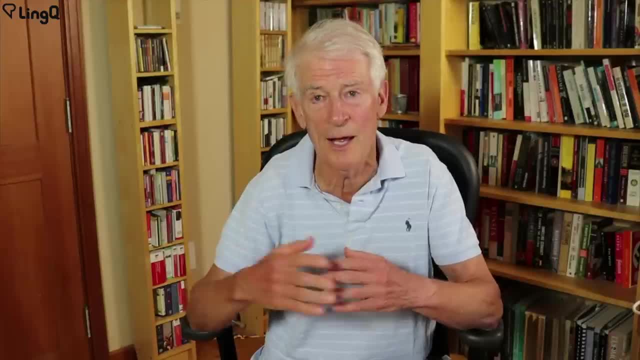 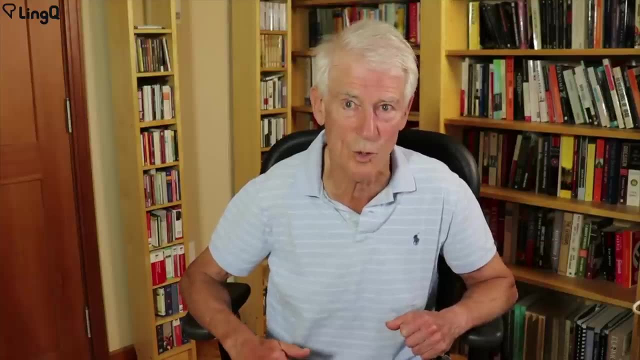 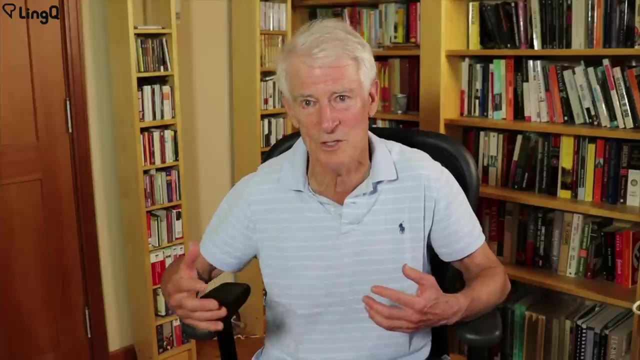 of a sweet spot. I'm acquiring enough new words. I'm not just reading material that has no meaning. However, if that sort of unknown words total is 30%, 25%, it's too difficult, It slows me down. I don't develop any genuine fluency in uh in the language. 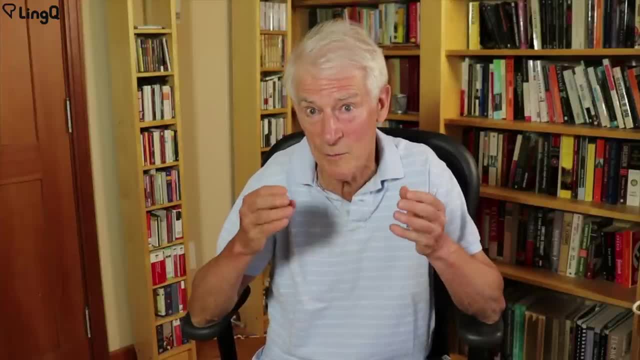 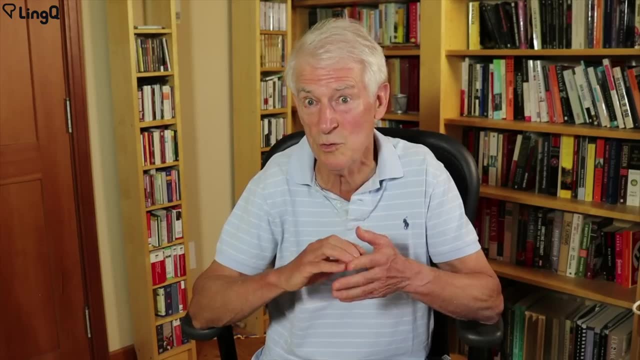 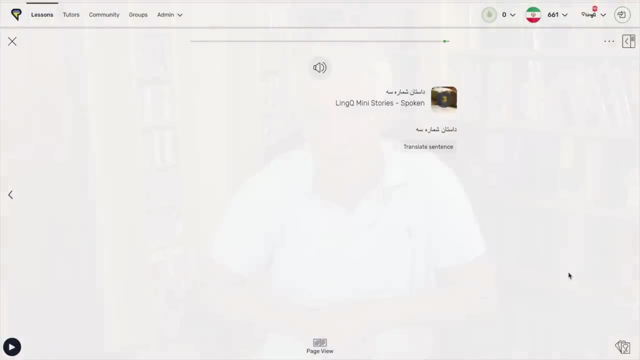 So to improve your reading comprehension, read more. increase your vocabulary, use audio, use tools. like you know the sentence view at LingQ, immerse yourself more in the language If there are structures that give you trouble, like some people complain that. 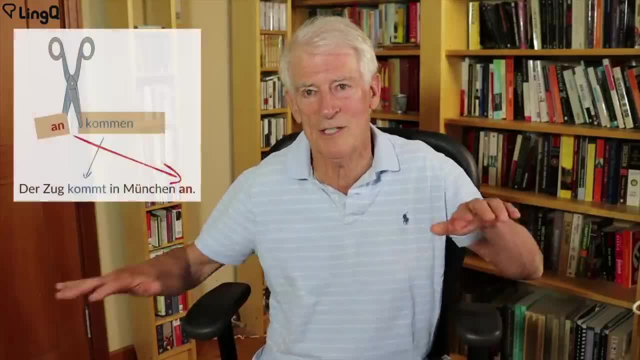 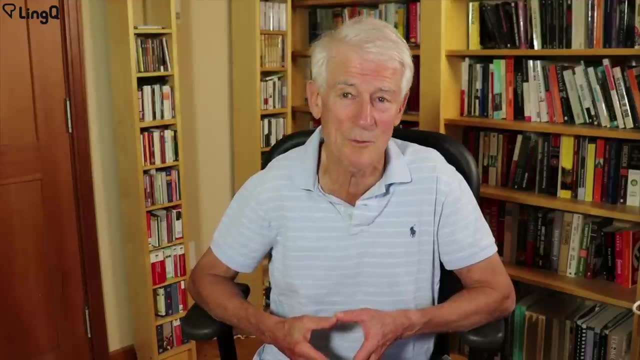 you know, in German you've got the separated verbs. uh, you know a lot long sentences with a verb comes at the end. or people reading in Japanese that find that, because that those languages are structured a little different, differently, It's difficult to read. 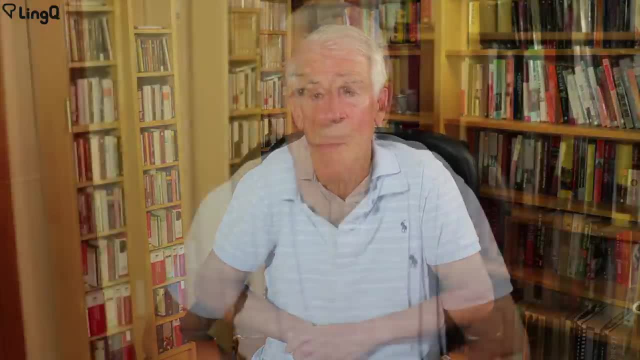 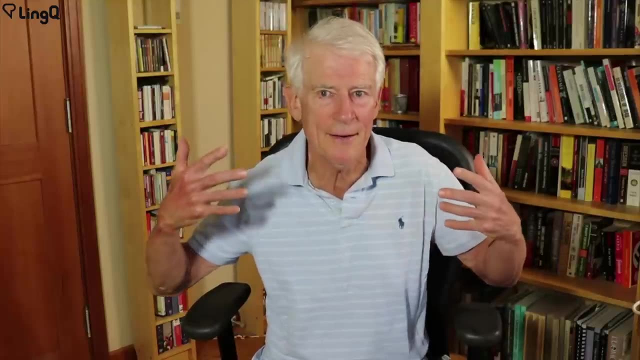 True, But that's all the more reason why you have to read more, And that's all the more reason why you have to listen more. And that's the only reason why you have to listen more, Because very often, when you hear those sentences spoken by the native speaker, 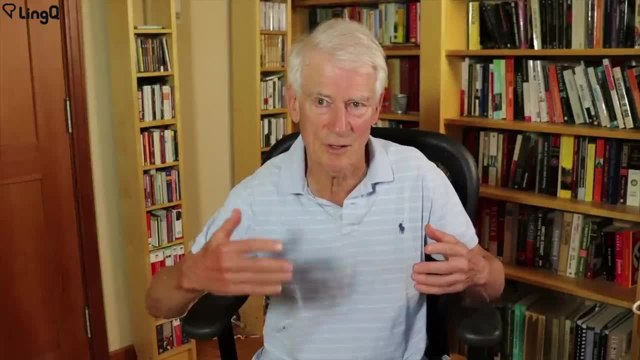 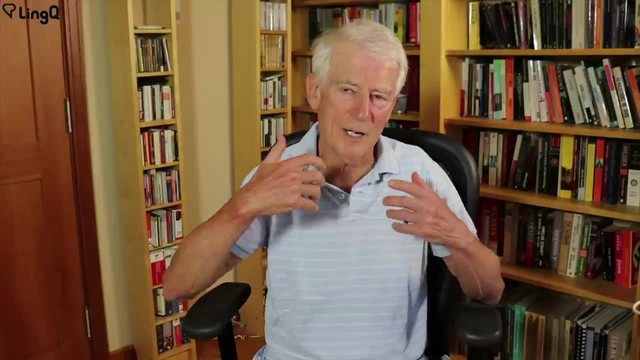 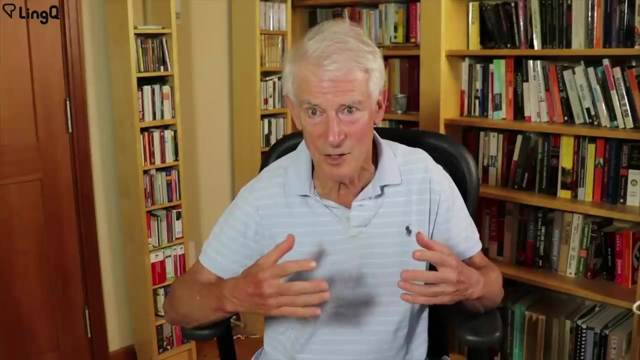 with a normal cadence, the normal intonation, the normal rhythm. it's easier to understand because the voice of the narrator, of the speaker, putting the emphasis in the right place, makes those sentences easier to understand When you don't have the benefit of that audio and you're just reading it. very